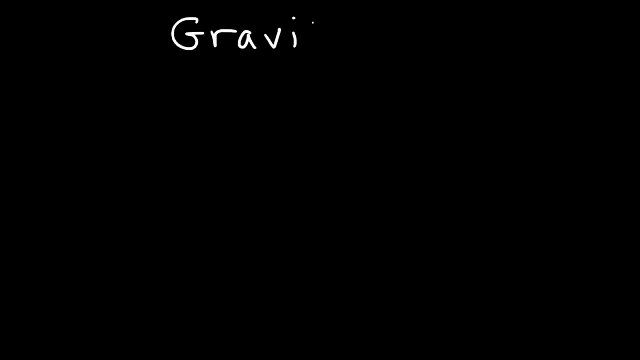 In this video we're going to talk about gravity. What is gravity? Gravity is a force that brings matter together. Now you know that if you place, let's say, a rock above the ground, you know that rock is going to fall towards the ground, And 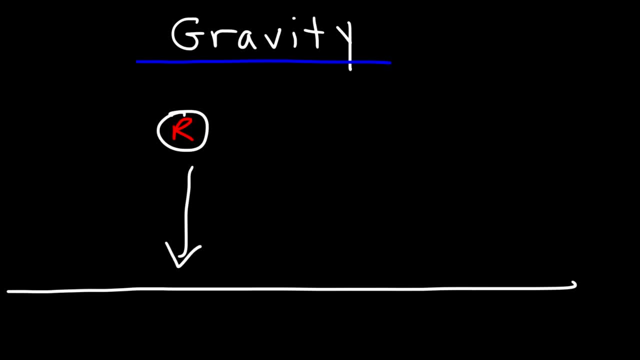 the reason for that is gravity. Gravity causes objects to fall. Now, gravity is a force, and that force brings the rock down towards the earth, But what you may not have known is that the earth actually accelerates towards the rock, However, because the mass of the earth is so much more greater than the rock. it 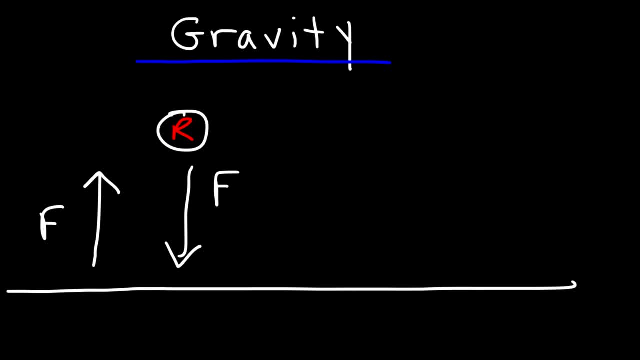 doesn't appear that the earth is moving. Its acceleration is insignificant Because the rocks mass is so small. it has a much larger acceleration And the rock it accelerates towards the ground at this rate- 9.8 meters per second squared. So this is known as 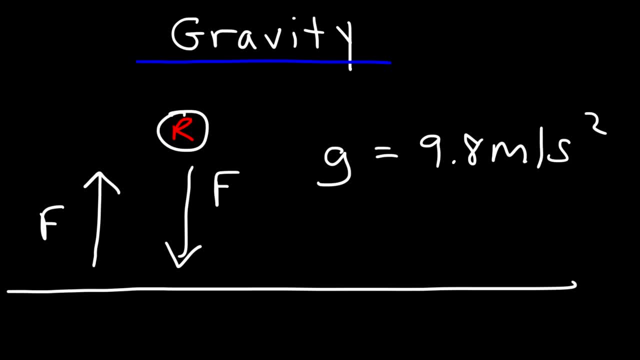 gravitational acceleration. This value tells us the rate at which the speed of the rock changes every second. So every second the velocity of the rock, it changes by 9.8 meters per second, So it's decreasing by 9.8 meters per second. 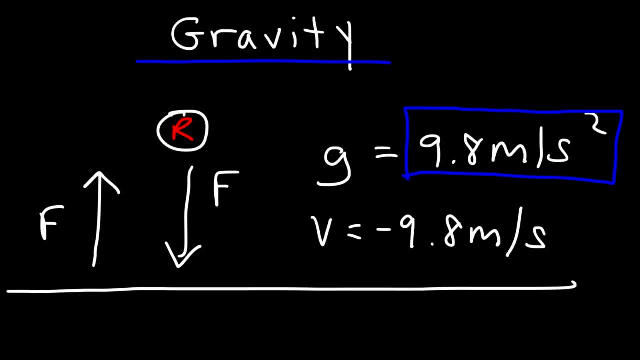 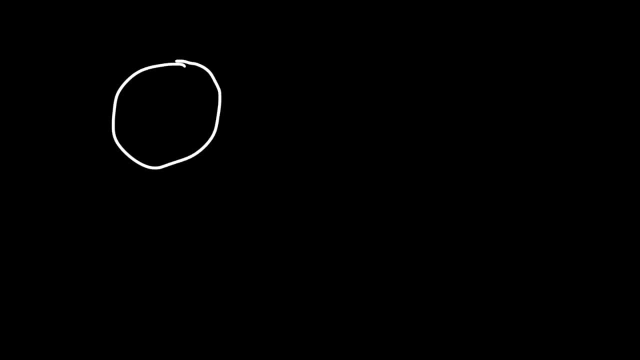 since it's going down in the negative y-direction. Now let's talk more about gravity. Let's say this is the earth And let's say this is the moon. Gravity brings matter together. The earth feels a force that accelerates it towards the moon, And 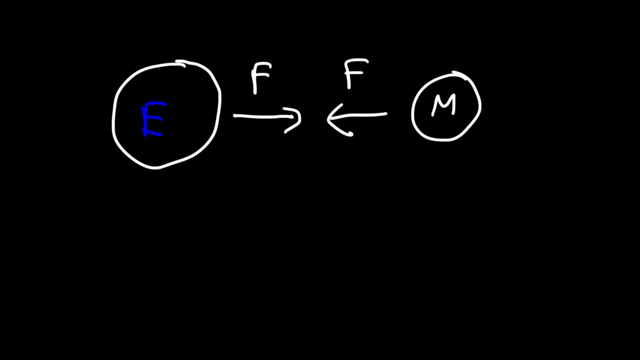 the moon feels an equal but opposite force that pulls it towards the earth, And so these forces, they have the same magnitude. And to calculate this force, it's equal to the gravitational constant times the mass of the earth times the mass of the moon, divided by the distance between their centers, which 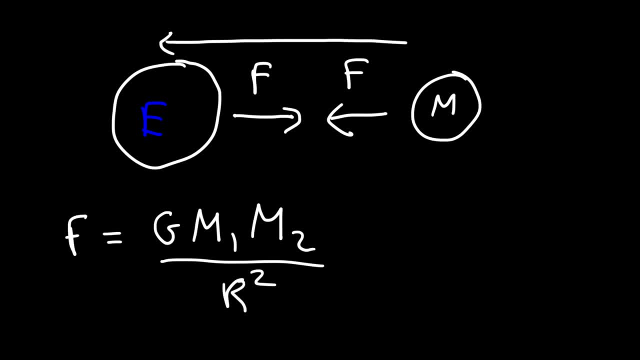 is r. So r is the distance between the center of the earth and the center of the moon, And so, using that equation, you can calculate the gravitational force between the earth and the moon. This equation is known as the universe's law of gravitation. so, as you can see, the force of gravity is proportional to the 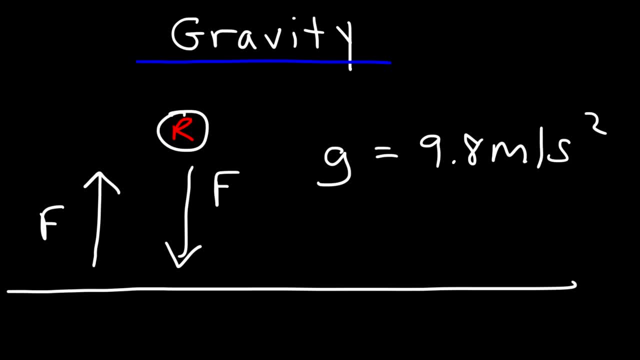 gravitational acceleration. This value tells us the rate at which the speed of the rock changes every second. So every second the velocity of the rock, it changes by 9.8 meters per second, So it's decreasing by 9.8 meters per second. 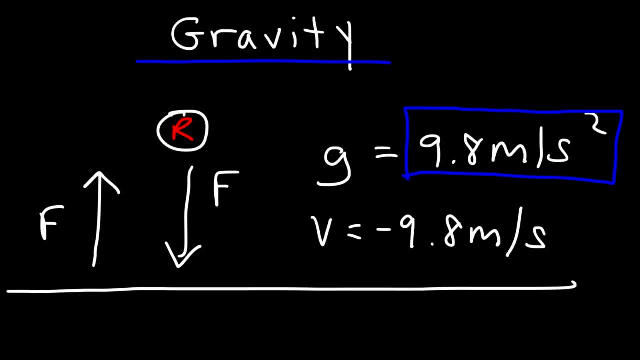 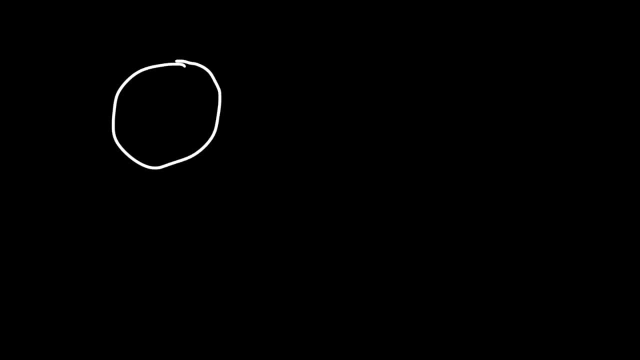 since it's going down in the negative y-direction. Now let's talk more about gravity. Let's say this is the earth And let's say this is the moon. Gravity brings matter together. The earth feels a force that accelerates it towards the moon, And 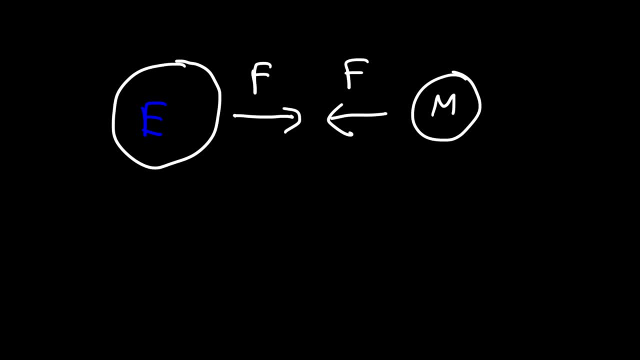 the moon feels an equal but opposite force that pulls it towards the earth, And so these forces, they have the same magnitude. And to calculate this force, it's equal to the gravitational constant times the mass of the earth times the mass of the moon, divided by the distance between their centers, which 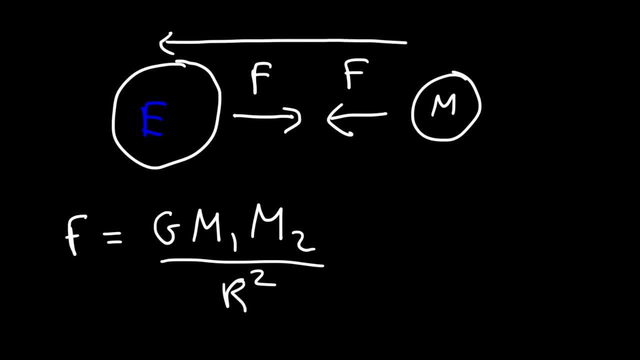 is r. So r is the distance between the center of the earth and the center of the moon, And so, using that equation, you can calculate the gravitational force between the earth and the moon. This equation is known as the universal equation, The universal law of gravitation. So, as you can see, the force of gravity is 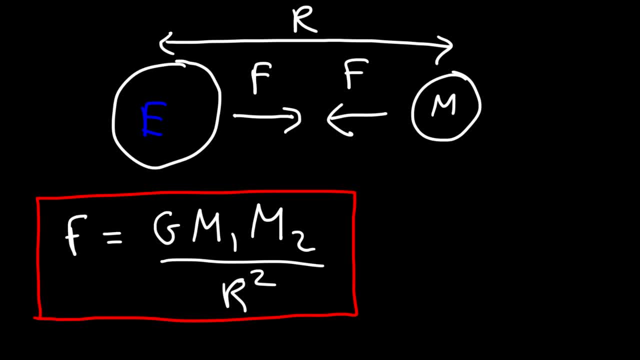 proportional to the masses of the two objects. For instance, let's say, if you have a rock and if you have, let's say, a book, The force of gravity between these two objects is not noticeable. The rock is not going to slide towards the book. 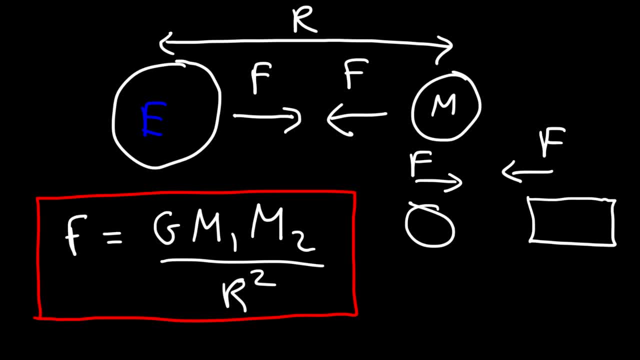 And the reason for that is because their masses are so small. For gravity to be significant, you need masses on a planetary scale. You need huge masses for it to be important. As you increase the mass of a planet, the gravitational force that it. 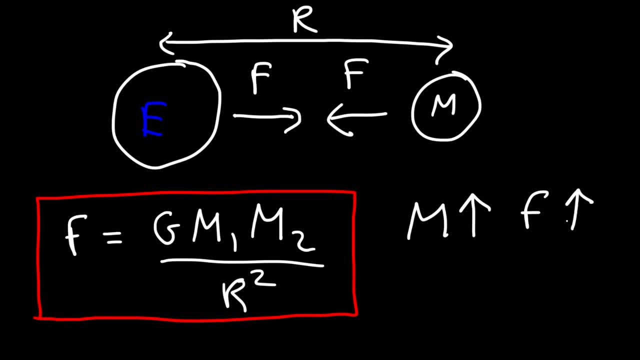 exerts on other planets increases. The second factor is distance. Notice that the distance is on the bottom of the equation. So as you increase the distance between a planet and another planet, the gravitational forces acting on those planets decreases. So the moon has a. 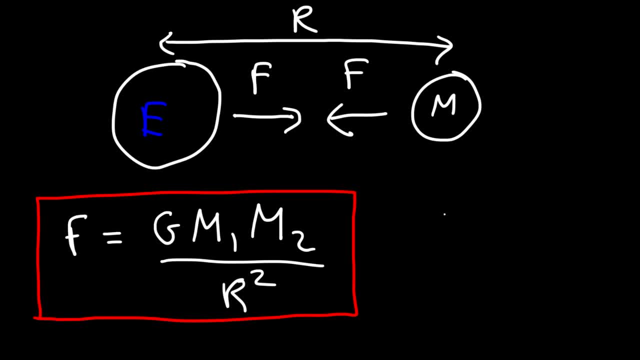 masses of the two objects. for instance, let's say, if you have a rock and if you have, let's say, a book, the force of gravity between these two objects is not noticeable. the rock is not going to slide towards the book, and the reason for that is because their masses are so small for gravity to be significant. you, 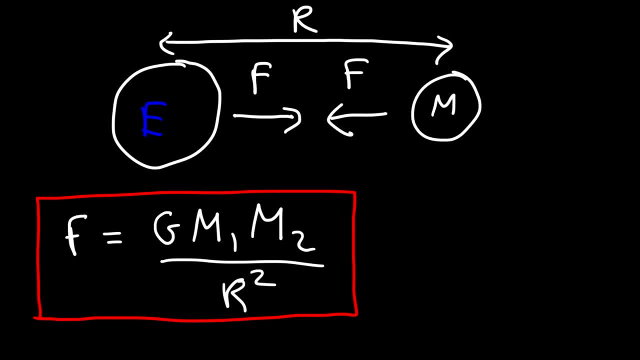 need masses on a planetary scale. you need huge masses for it to be important. as you increase the mass of a planet, the gravitational force that it exerts on other planets increases. the second factor is distance. notice that the distance is on the bottom of the equation. so as you increase the distance, 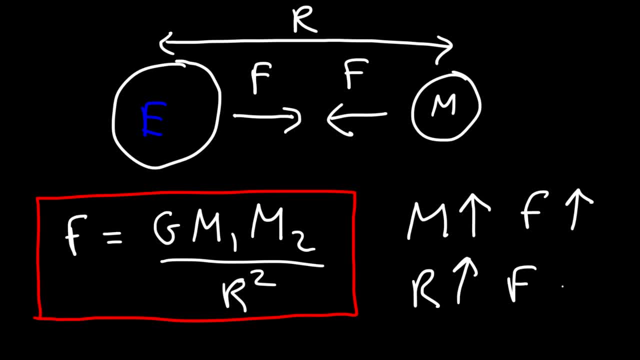 between a planet and another planet, the gravitational forces are acting on those planets decreases. so the moon has a greater effect on planet earth compared to Pluto, because Pluto so far away, so gravity plays a role on objects that are nearby. objects that are far away, gravity weakens greatly in. 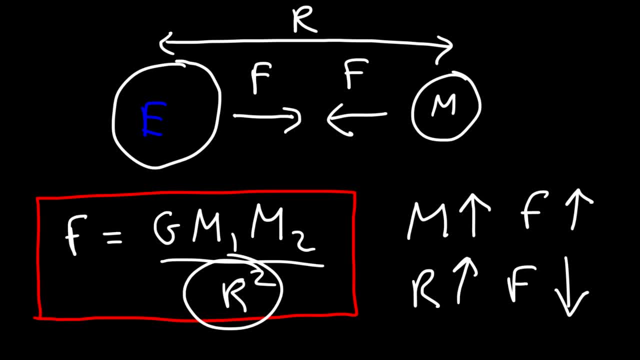 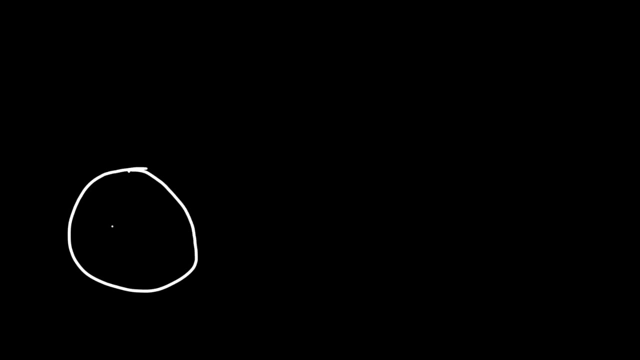 fact, as you double the distance between two planets, the gravitational force reduces by a factor of four. if you double one of the masses of the planets, the gravitational force will double. now it turns out that the gravitational force is the same as the weight force, and let me illustrate that. so let's say this is the earth and let's 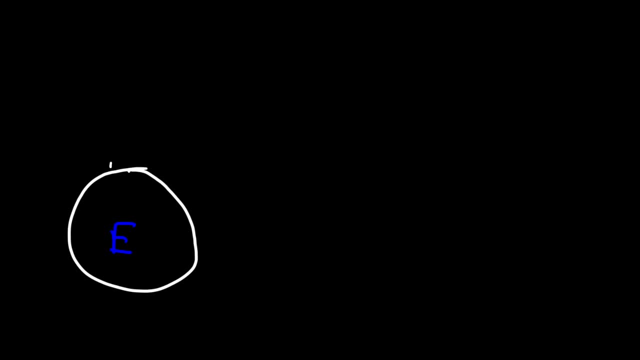 say we have a 20 kilogram block resting on the earth. now what is the weight force of that 20 kilogram block? the weight force is simply the mass times the gravitational acceleration. so it's going to be the mass of the block, which is 20 kilograms times the gravitational acceleration of. 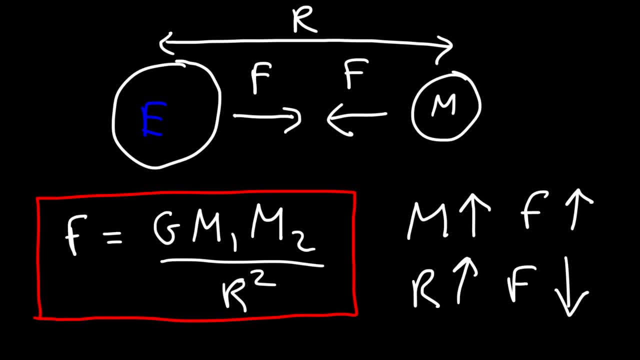 greater effect on planet Earth compared to Pluto, because Pluto is so far away. So gravity plays a role on objects that are nearby. Objects that are far away, gravity weakens greatly. In fact, as you double the distance between two planets, the gravitational force reduces by two. 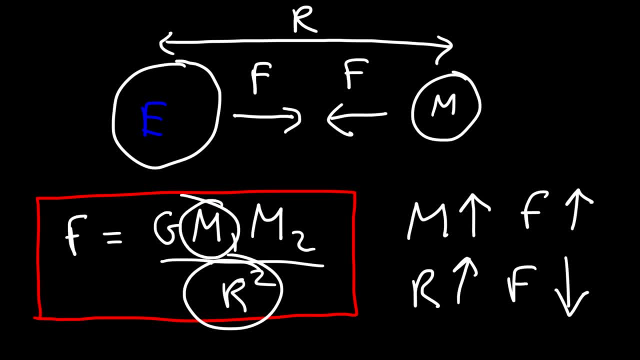 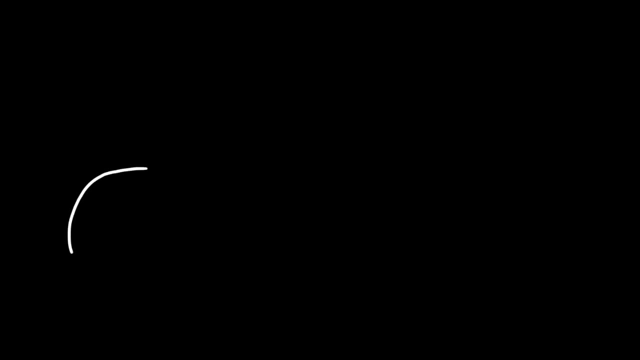 By a factor of four. If you double one of the masses of the planets, the gravitational force will double. Now it turns out that the gravitational force is the same as the weight force, And let me illustrate that. So let's say this is the 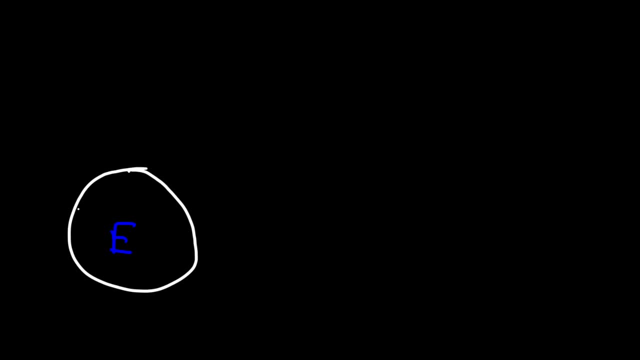 Earth. And let's say we have a 20 kilogram block resting on the Earth. Now what is the weight force of that 20 kilogram block? The weight force is simply the mass times the gravitational acceleration. So it's going to be the mass of the block, which is 20 kilograms times the 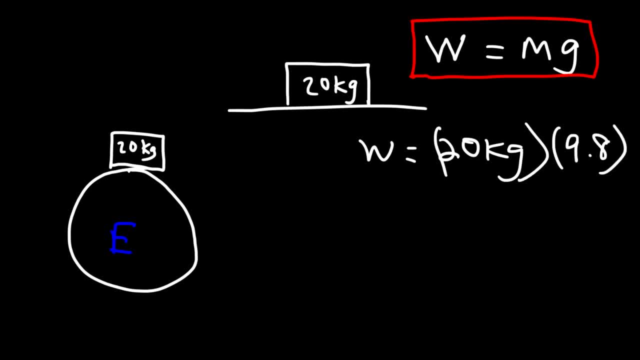 gravitational acceleration of 9.8 meters per second. squared So 20 times 9.8, that gives us a weight force of 196 newtons. Now let's see if we can get the same answer using the universal law of gravitation formula. So the formula was F. 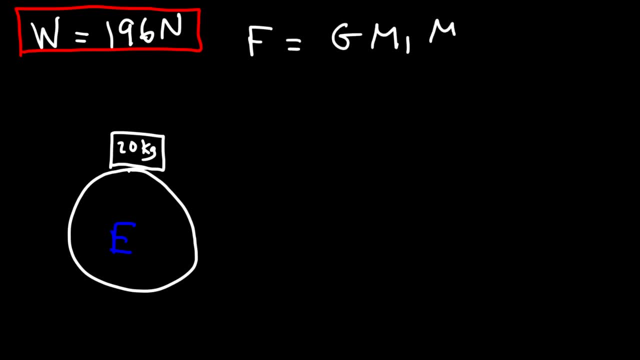 is equal to G, M1 M2 over R squared. Now, G is the universal gravitation constant, which is 6.2.. So that's 5.67 times 10 to the negative 11.. And it's newtons times square meters. 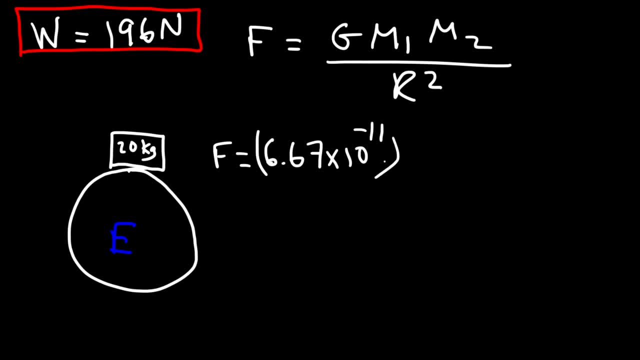 divided by square kilograms Now, the mass of the Earth, that's 5.98 times 10, to the 24 kilograms, The mass of the block M2, is 20 kilograms, And the distance between the center of the Earth and the surface of the Earth, because the block is on the 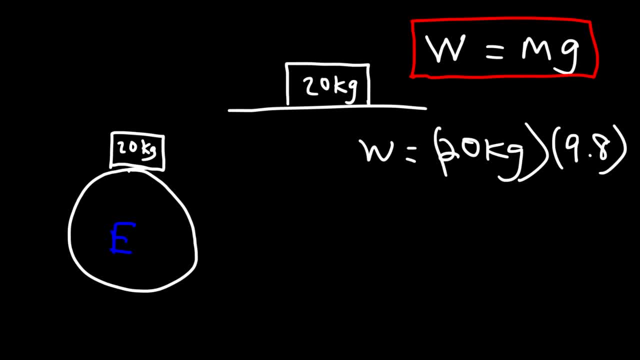 9.8 meters per second square. so 20 times nine point eight, that gives us a weight force of 196 N. Now let's see if we can get the same answer using the universal law of gravitation formula. So the formula was: F is equal to g, m1 m2 over r squared. 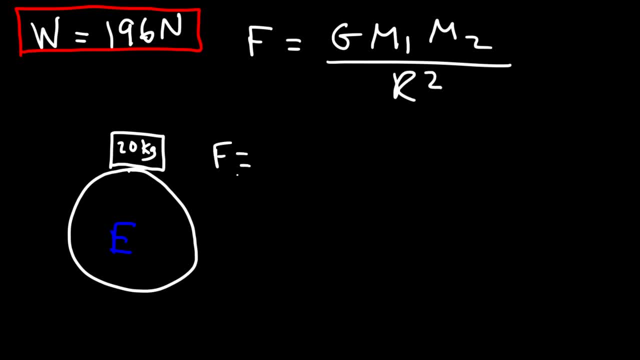 Now, g is the universal gravitation constant, which is 6.67 times 10 to the negative 11, and it's newtons times square meters divided by square kilograms. Now the mass of the earth, that's 5.98 times 10 to the 24 kilograms. The mass of the block m2 is 20 kilograms. 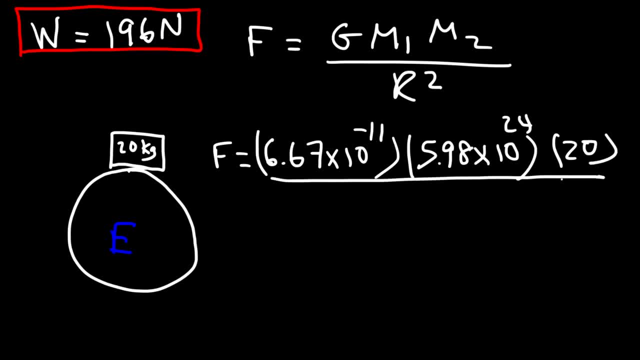 and the distance between the center of the earth and the center of the earth is 5.98, and the surface of the earth, because the block is on the surface. that's the radius of the earth, which you can call r? e and you can look up this value in a textbook: It's 6.38 times. 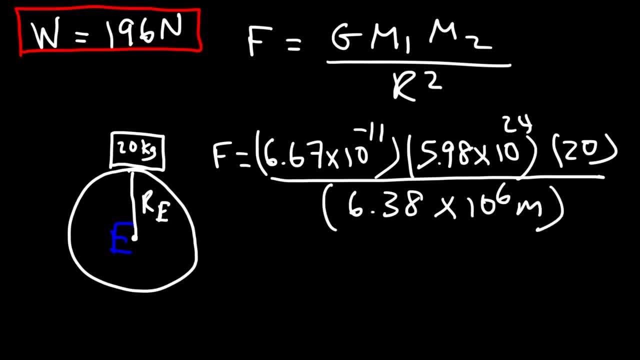 10 to the 6 meters, and we need to square it. So go ahead and type these numbers into your scientific device. Give me a few seconds. I'm almost done. So the answer that I got is 195.98 newtons. So 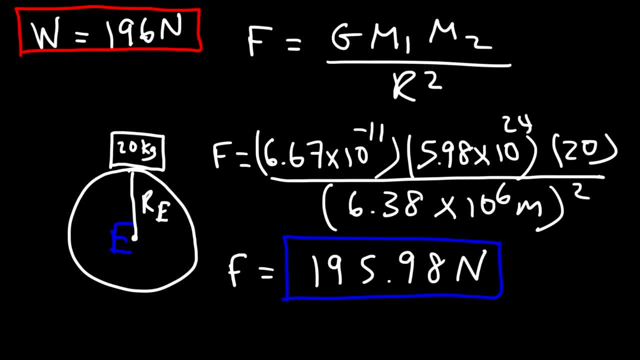 as you can see, the gravitational force, or the weight force, is about 196 N. Now, of course, these numbers that I'm using are rounded figures, so that's why it's not exactly the same, but it should be the same. So this is approximately 196 N. 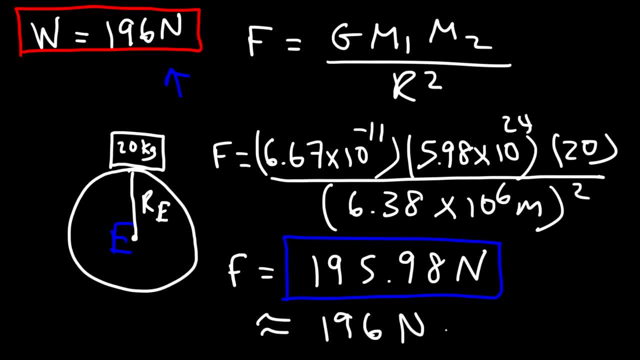 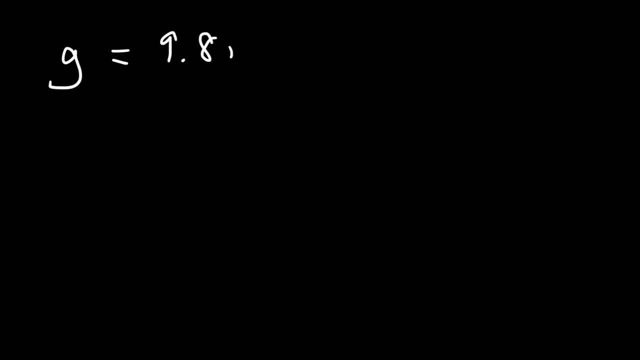 So that's why it's not exactly the same, but it should be the same. So this is approximately 196 N Newton's. So the weight force and gravity, or the gravitational force, they're identical. Now how do we get this number? How do we calculate the gravitational? 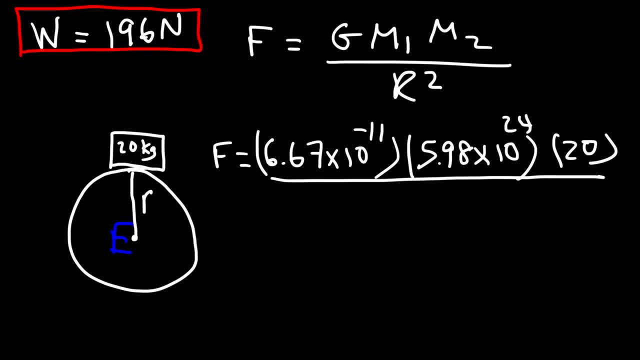 surface. that's the radius of the Earth, which you can call Re, And you can look up this value in a textbook. It's 6.38 times 10 to the 6 meters, And we need to square it. So go ahead and type these numbers into your scientific device. 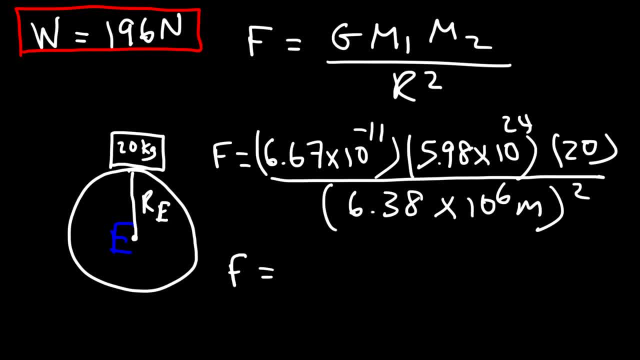 Give me a few seconds. I'm almost done. So the answer that I got out of this experiment is which one would be greater or greater than The answer is A. So where is that elementary saving quieren Rate function in this problem Here? 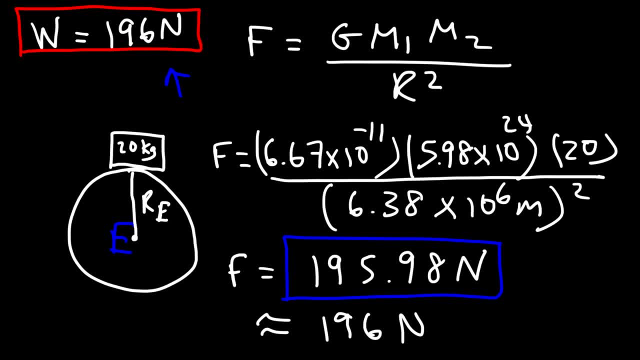 If O is greater than 0.. What's myamour? A, P, T, C, P, C, R, R, P, P or the gravitational force? they're identical. Now, how do we get this number? 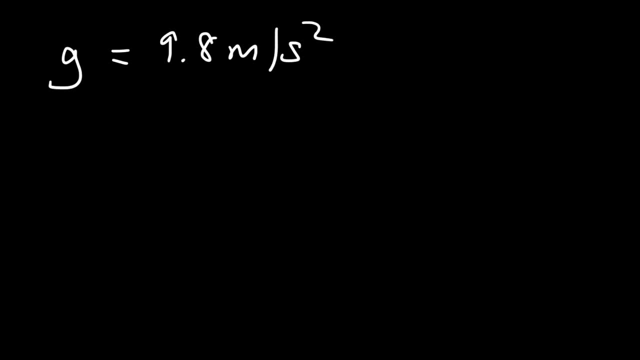 How do we calculate the gravitational acceleration? Well, let's look at these two equations. The weight force is mg and the force of gravity is gm1m2 over r squared. Now we said that these two they're the same, which means that we can set these two portions of the equation equal to each other. 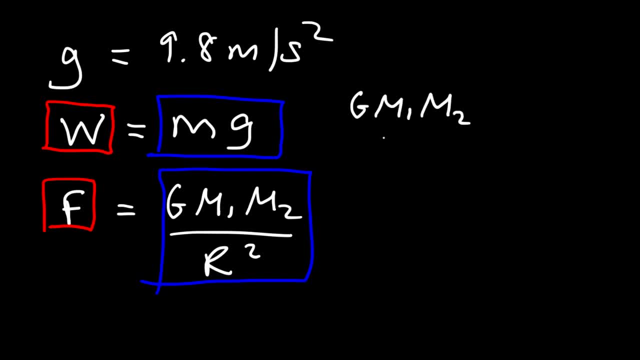 So let's do that. gm1 over m2, I mean times m2 over r squared, Let's set it equal to mg. Now all we need to do is cancel one of the masses Particularly. it really doesn't matter which mass you cancel, m1 or m2.. 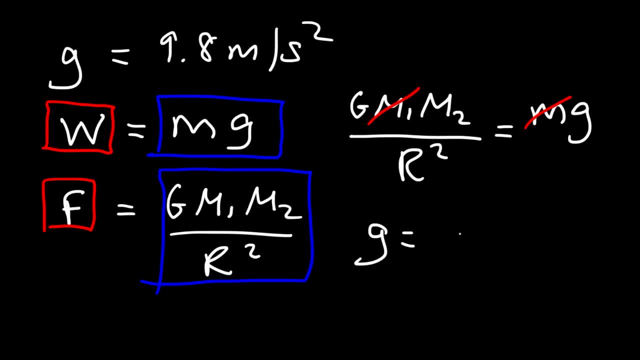 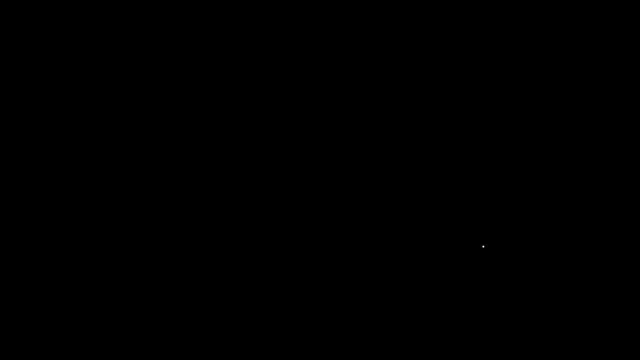 So the gravitational acceleration of a planet is the gravitational constant times the mass of the planet over r squared. So let's calculate it for the Earth. So we're going to use the mass of the Earth and the radius of the Earth. So g is 6.67 times 10 to the minus 11.. 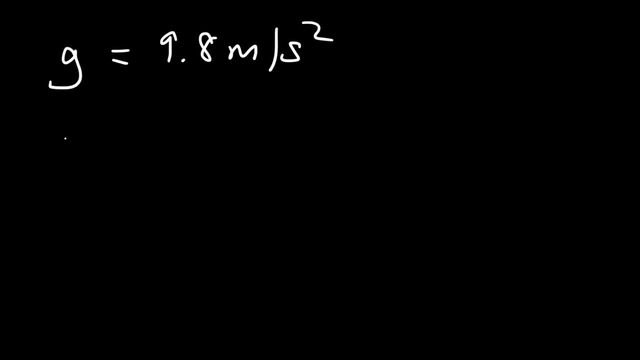 acceleration. Well, let's look at these two equations: The weight force is mg and the force of gravity is gm1m2 over r-squared. Now we said that these two they're the same, which means that we can set these two portions of the equation. 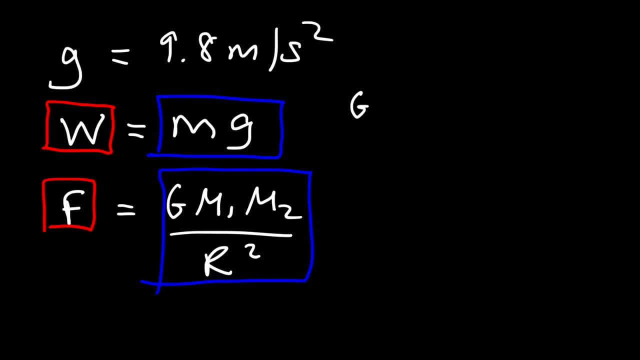 equal to each other. So let's do that. gm1 over m2, I mean times m2 over r-squared. Let's set it equal to mg. Now, all we need to do is cancel one of the masses. Now, all we need to do is cancel one of the masses. 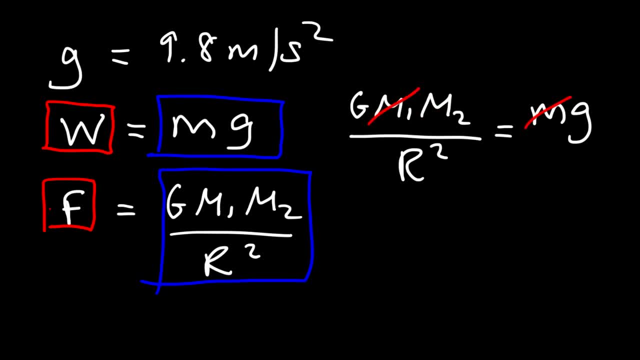 So let's do that gm1m2 over r-squared. Now all we need to do is cancel one of the masses Particularly. it really doesn't matter which mass you cancel, m1 or m2.. So the gravitational acceleration of a planet is the gravitational constant times, the 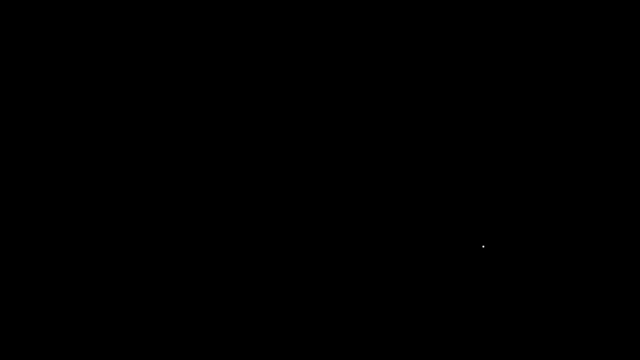 mass of the planet over r-squared. So let's calculate it for the Earth. So we're going to use the mass of the Earth and the radius of the Earth. So g is 6.6, 7 times 10 to the minus 11.. The mass of the Earth: we said it's 5.98 times 10 to the 24. 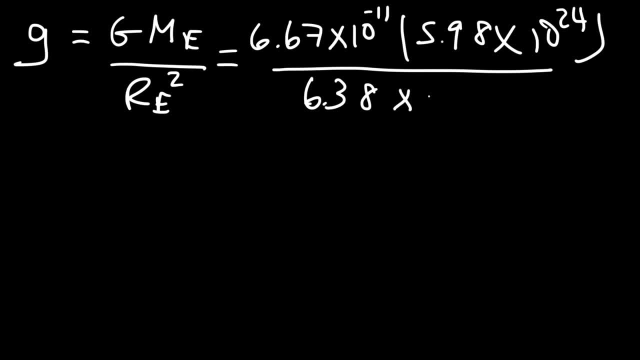 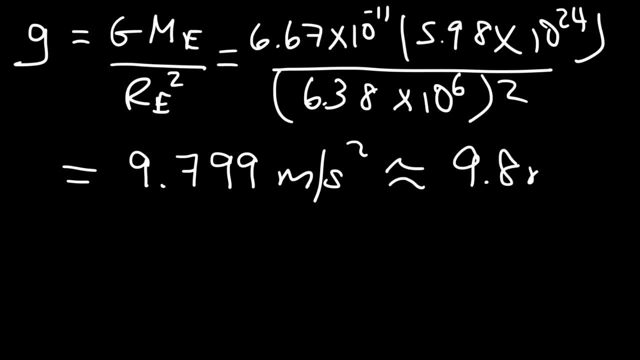 squared, which you can round that to 9.8 meters per second squared, And so this formula helps us to calculate the gravitational acceleration of any planet. It could be a moon, it could be a planet, it could be a star like the Sun. 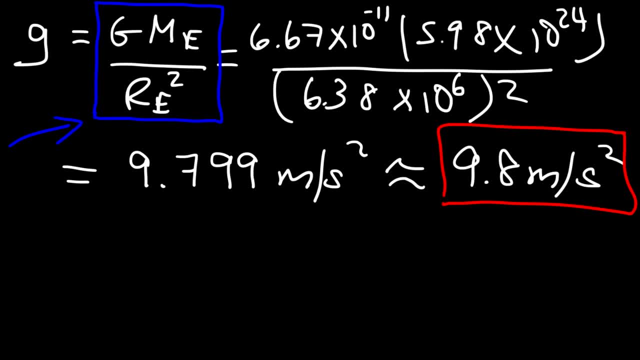 You can use this to calculate the gravitational acceleration of any object. Now, that's basically it for this video. That's all I got. So if you like this video, feel free to subscribe to this channel and don't forget to click on that notification. 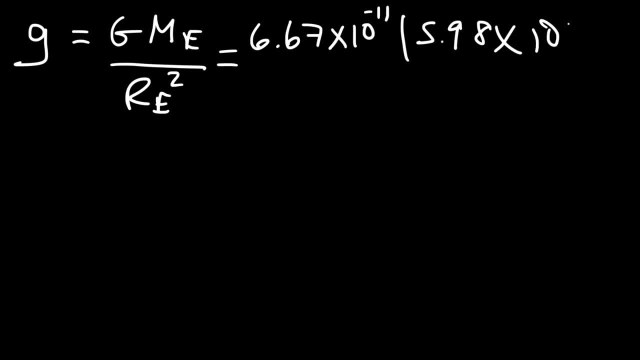 The mass of the Earth we said it's 5.98 times 10 to the 24 kilograms, And the radius of the Earth is this number again in meters. So go ahead and type that in, So you should get 9.799 meters per second squared. 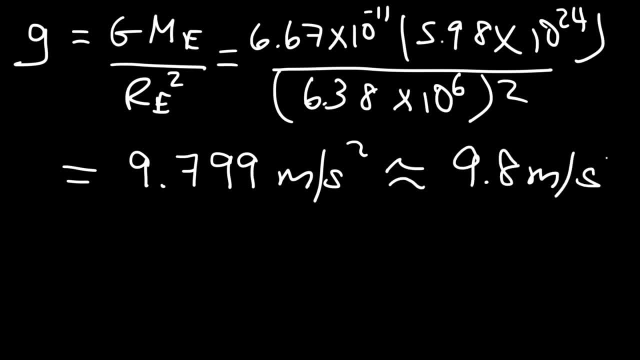 which you can round that to 9.8 meters per second squared, And so this formula helps us to calculate the gravitational acceleration of any planet. It could be a moon, it could be a planet, it could be a star like the sun. 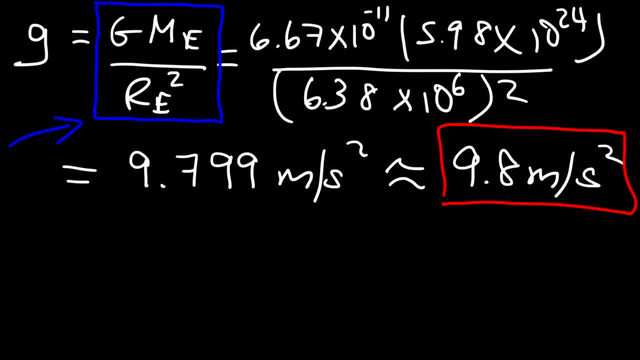 You can use this to calculate the gravitational acceleration of any object. Now, that's basically it for this video. That's all I got. So if you like this video, feel free to subscribe to this channel And don't forget to click on that notification bell. 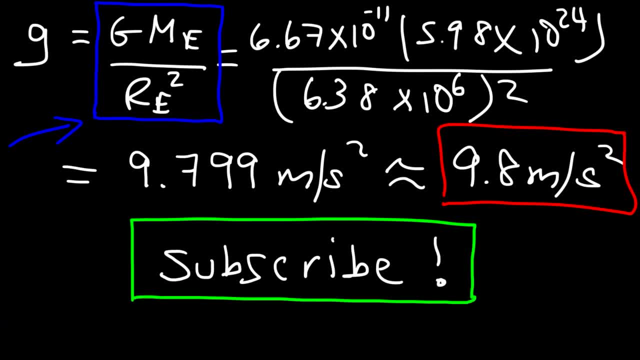 In addition, for those of you who are new to this channel and those of you who want more math problems on gravity and the Universal Law of Gravitation, I have another video that has a lot of problems that you can work on, And what I'm going to do is I'm going to post a few links in the description section of this video. 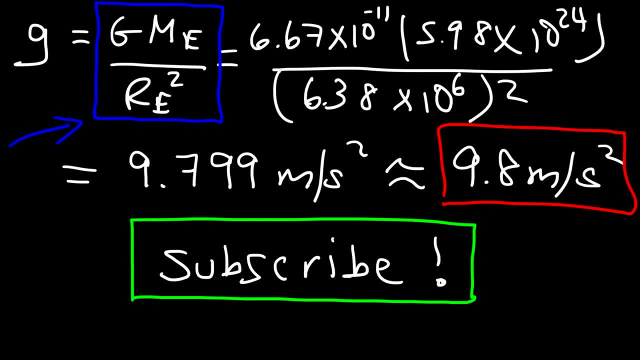 that will point you towards more problems like finding the gravitational force, finding the distance between planets and stuff like that. You'll see it, And not only that. I'm going to have some other topics related to gravity, like how to find the speed of a satellite in orbit. 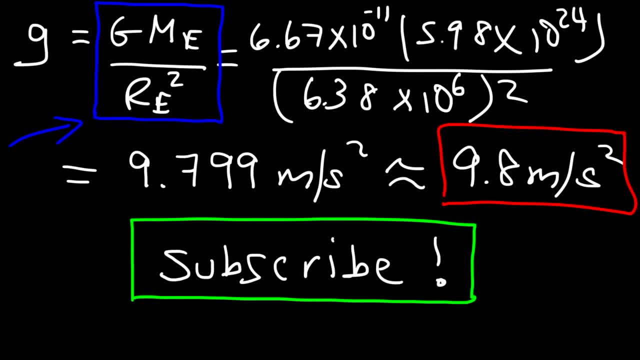 and some other problems on centripetal force and Kepler's third laws and just other topics that relate to gravity, space and planets and things like that. So when you get a chance, feel free to check out those links below. 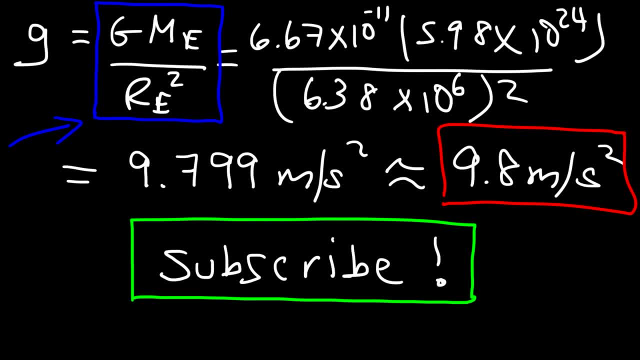 And whatever you do, don't forget to subscribe to this channel. Now I do have other topics besides physics. I do have a playlist on physics. You can check out my playlist. It's on my channel if you want more info on that.